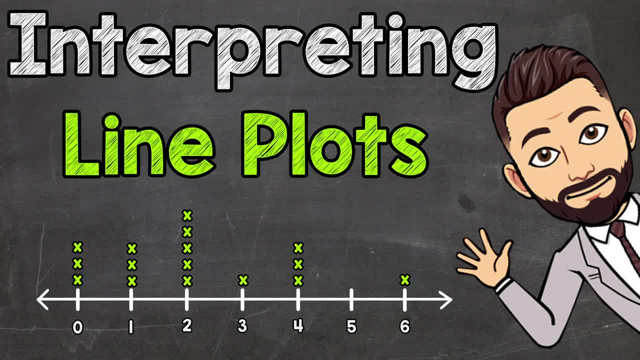 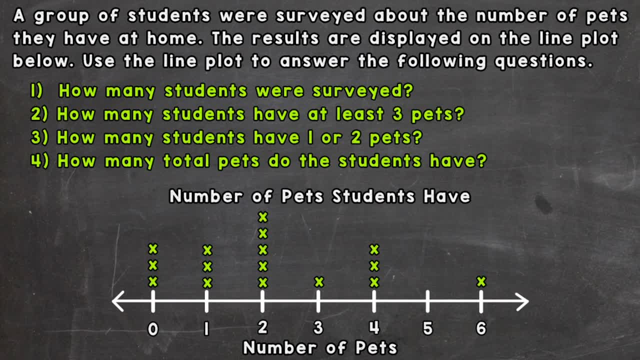 Welcome to Math with Mr J. In this video we're going to take a look at a line plot and interpret or read the results of that line plot. So let's take a look at the situation up top. A group of students were surveyed about the 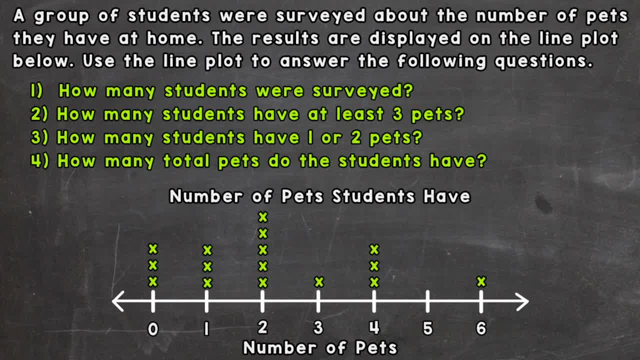 number of pets they have at home. The results are displayed on the line plot below. Use the line plot to answer the following questions. So, number one: how many students were surveyed? Well, let's take a look at our line plot here and see what this line plot tells us. Well, the title tells us what it's about, right? 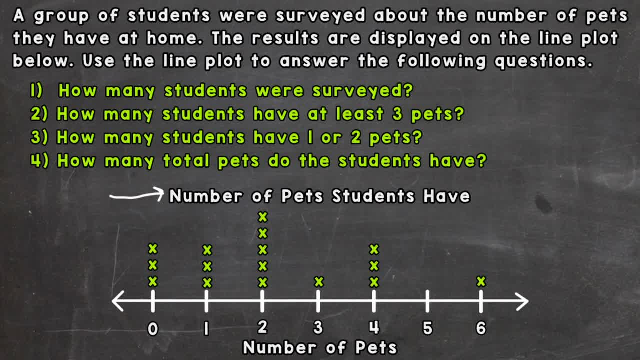 It's the number of pets students have, and these numbers down here represent the number of pets. So how many students were surveyed or being surveyed by the number of pets was the answer? Slide 1.. As the our line plot explains it to the audience of the slide practice: 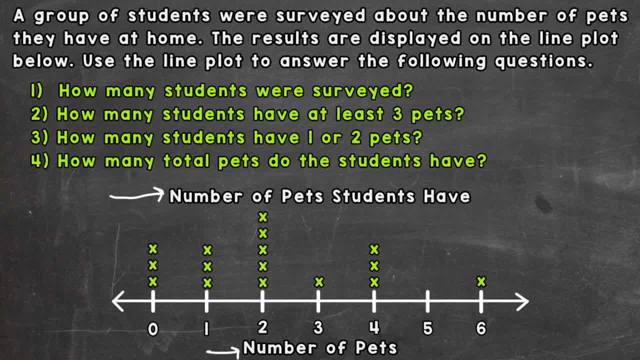 We need to count the number of X's in the line plot here, because each X represents a student that was surveyed. So here we have: for 0 we have 3,. for 1 we have 3,, for 2 we have 5,. for 3 we have 1,. for 4 we have 3 students and for 6 we have 1 student. 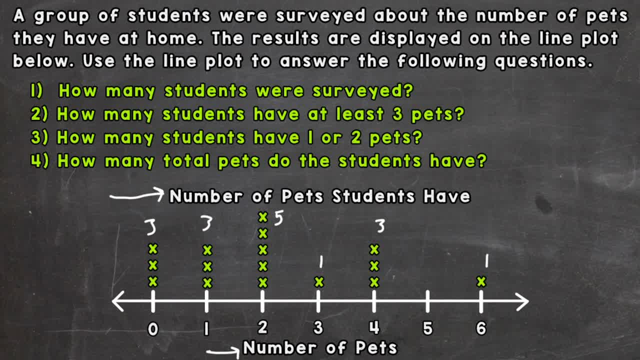 5, there's nothing there. there aren't any X's, so no students within that survey had 5 pets, And that's okay if you don't have X's above all of the numbers. So how many total students is that? 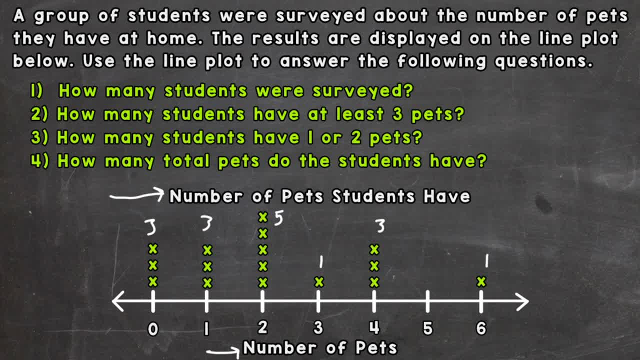 Well, 3 plus 3 is 6, plus 5 is 11,, plus 1 is 12,, plus 3 is 15,, plus 1 is 16.. So how many students? Well, 16 students. We counted the total number of X's and remember, each X represents a student. that was part of that survey. 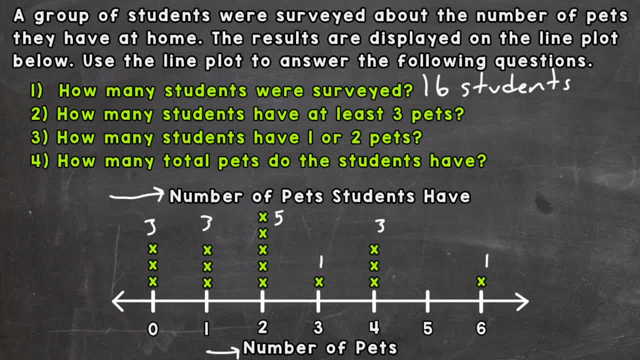 So number 2, how many students have at least 3 pets? So at least means 3 or more, so we include 3.. So let's see Well, for 3 or more, at least 3.. We need to look at this portion of the line plot. 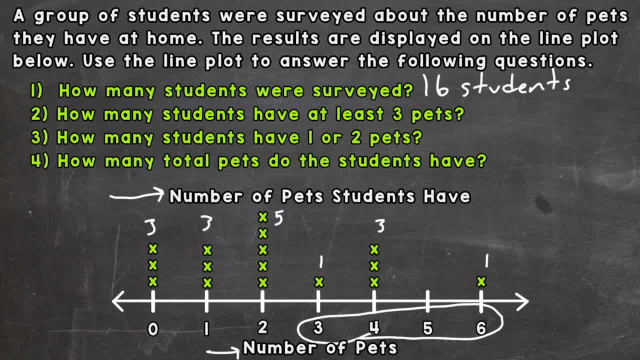 So we have 1 here for 3 pets, 3 for 4, and 1 for 6.. So that is a total of 5 students. Number 3,: how many students have 1 or 2 pets? So we need to take a look at this portion of our line plot. 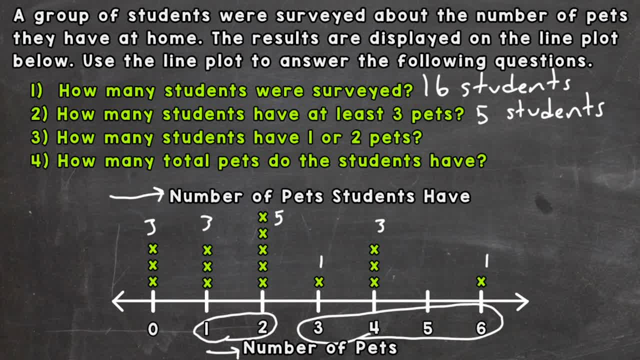 1 or 2.. So 3 students have 1 pet and 5 students have 2 pets, So that's a total of 8 students. And lastly, this is probably the most difficult question out of the 4.. 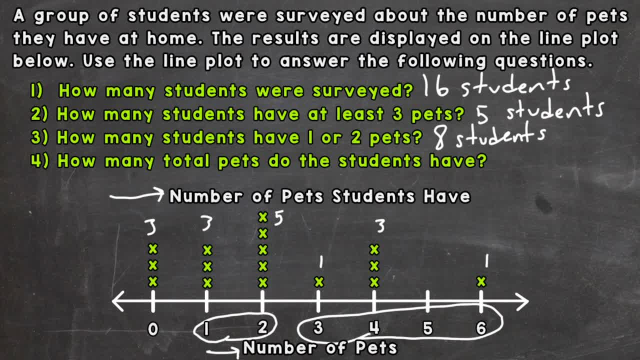 How many total pets do the students have? This is not a matter of just counting up all of the X's, Because each X- for example, right here, each X- holds a value of 0. Because each of those students have 0 pets. 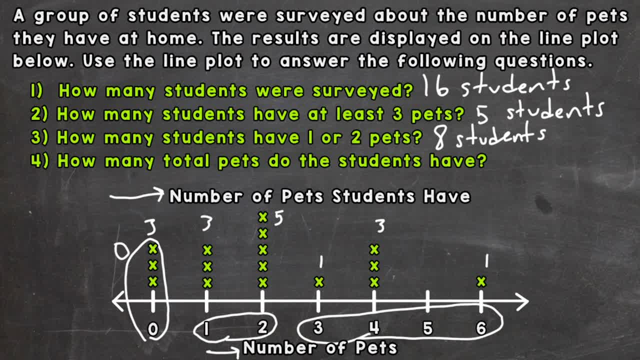 So this is 0 right here. This is going to be worth 0 for that question. Here for 1 pet: right, we have 3 students that have 1 pet, So those X's represent a value of 1.. 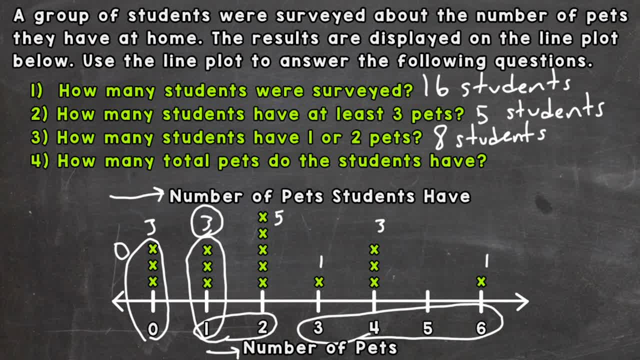 So I'm going to circle, I'm going to circle this. 3, so we know that the value of that part of the graph is 3.. Now, 2 pets: here we have 5 students that have 2 pets at home. So how many total pets is that? 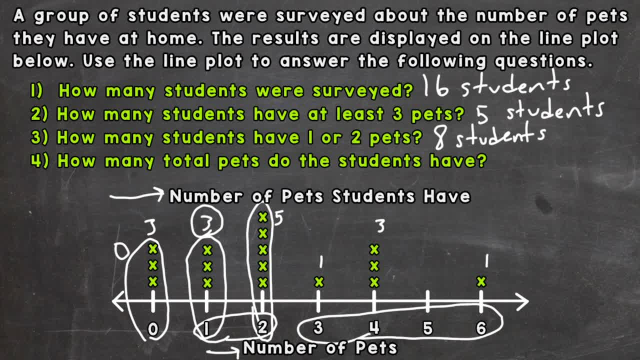 It's not 5, it's actually 10. Because, again, each of those 5 students have 2 at home, So this is going to be 10.. Then, for 3 pets, we have 1 student with 3 pets. 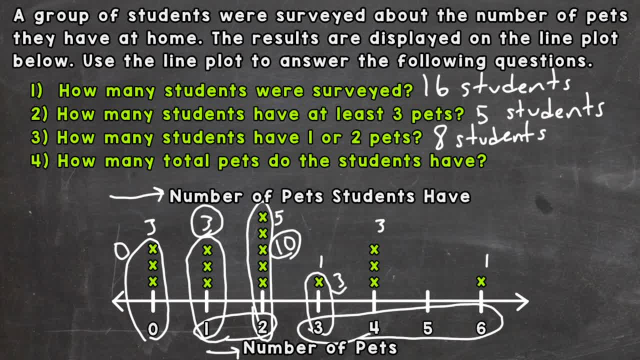 So the value of that X in terms of pets is 3.. 4 pets: well, 3 students have 4 pets, So that's a total of 12.. And then, lastly, we have 1 student with 6 pets.